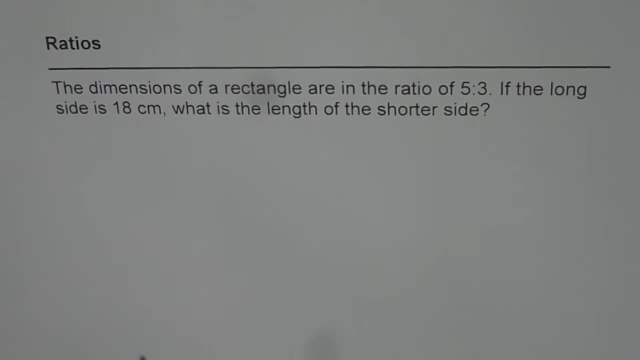 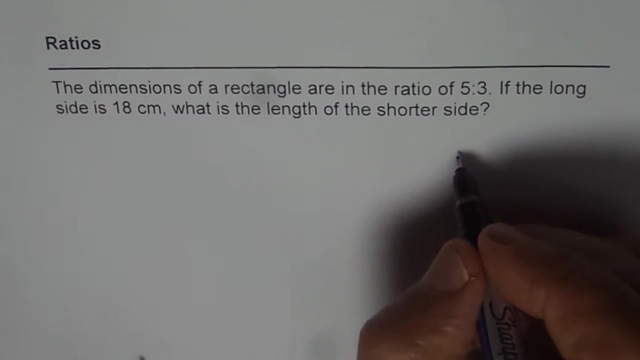 I'm Anil Kumar and here is an interesting question on ratios. The dimensions of a rectangle are in. the ratio of 5 is to 3.. If the long side is 18 centimeter, what is the length of the shorter side? Okay, so let's construct one rectangle here, And what we are saying? 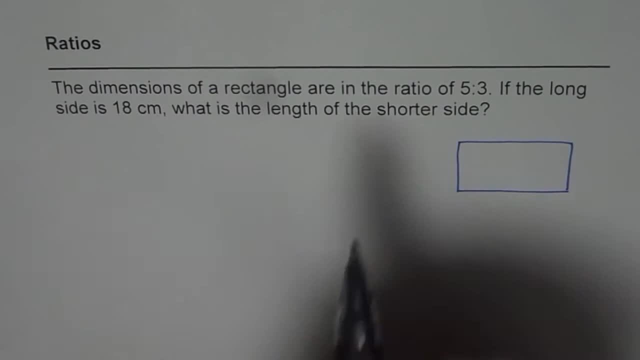 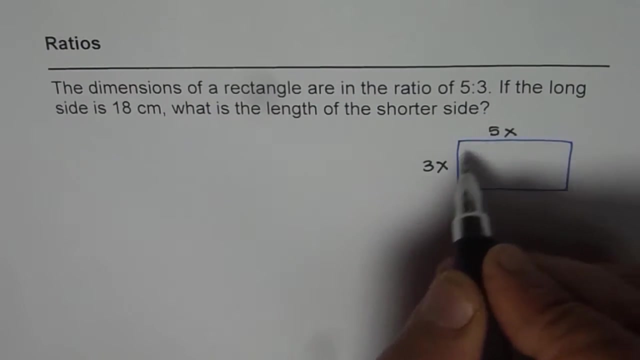 is that the sides are in the ratio of 5 is to 3.. So in that case, if I say one side is 3 times x, the other side should be 5 times x. That is what it means when I say that the 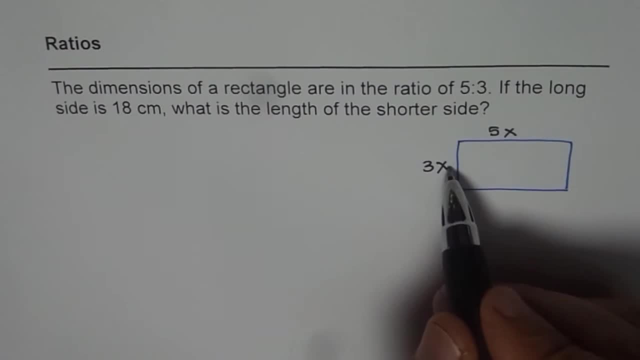 two sides are in the ratio of 5 is to 3.. Do you understand? That is kind of very critical to understand. If you understand that, then the question is so simple. The dimensions of a rectangle are in the ratio of 5 is to 3.. So that means 5 over 3. 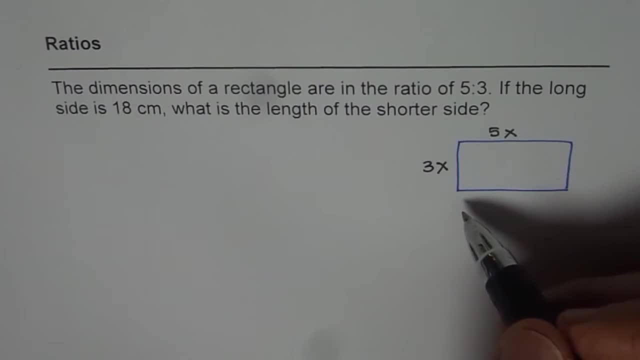 is a constant and let that be x, So anything. So 5x and 3x, that is, the ratio of 5 is to 3.. If the long side is 18 centimeter, what is the length of the shorter side? That is, 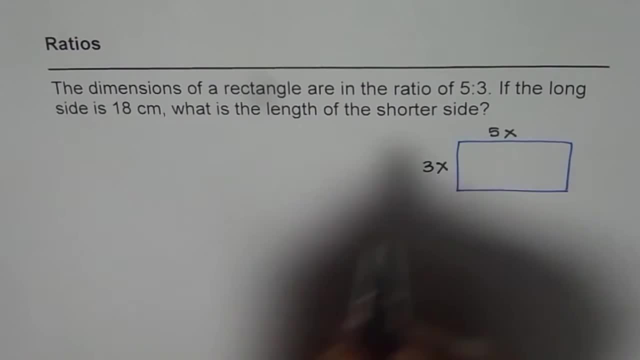 the question right. So what we have here is long side is 5x. So if the long side is 6, that means we have long side 5x. So we have long side 5x equals to 18.. That means 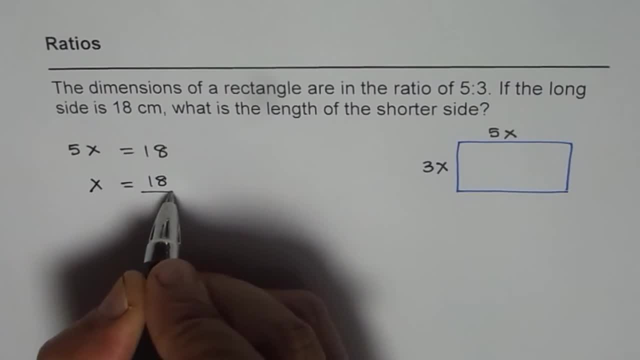 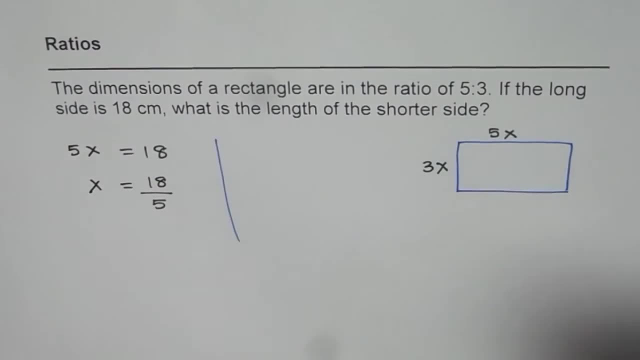 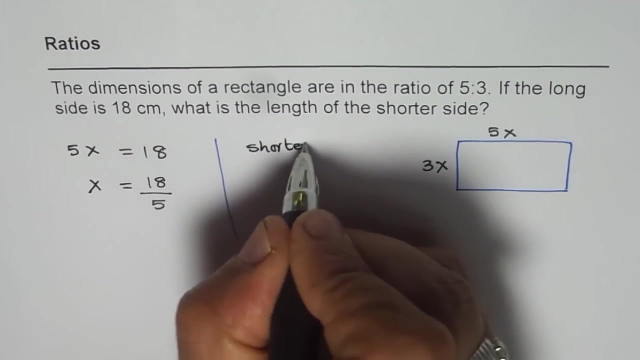 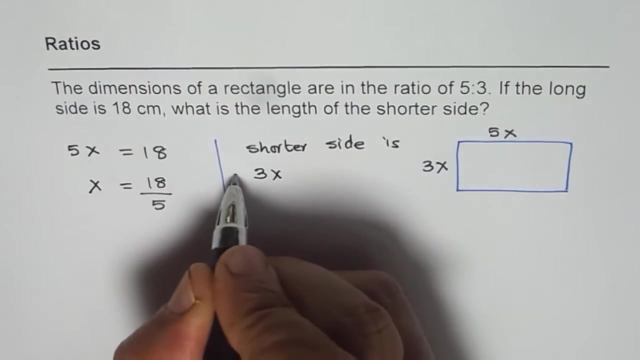 x is equal to 18 divided by 5, correct? So what is the shorter side? Shorter side is 3 times x, 3 times x, right? So shorter side is 3 times x, 3 times x. right Is equal to. 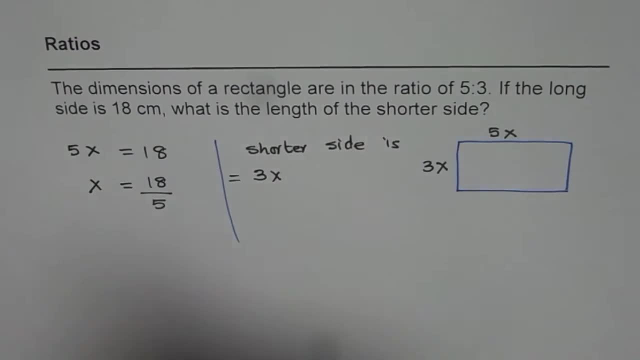 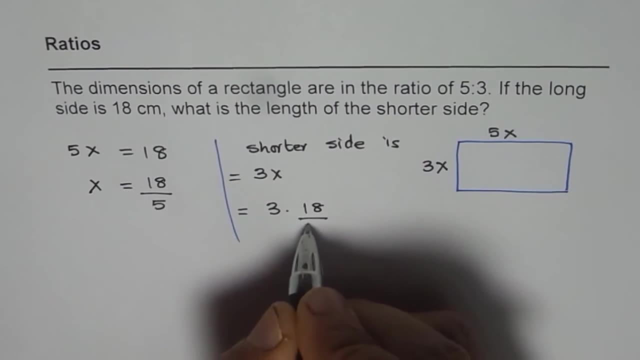 times x, but x is 18 over 5, correct? Therefore, we can replace this x with 18 over 5.. So we get 3 times 18 over 5.. Do you understand? So that is the length of the shorter side.